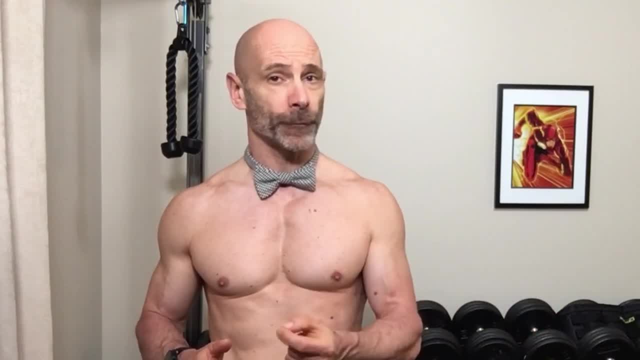 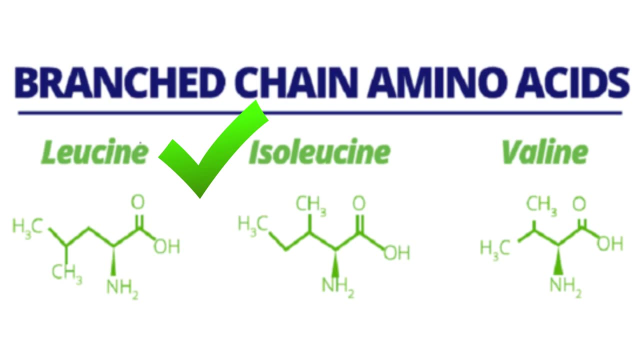 significant role than all the others. We must get enough in our food to maximally stimulate muscle protein synthesis. Leucine is one of three branched chain amino acids that are known to stimulate muscle protein synthesis. These amino acids can be used to stimulate muscle protein. 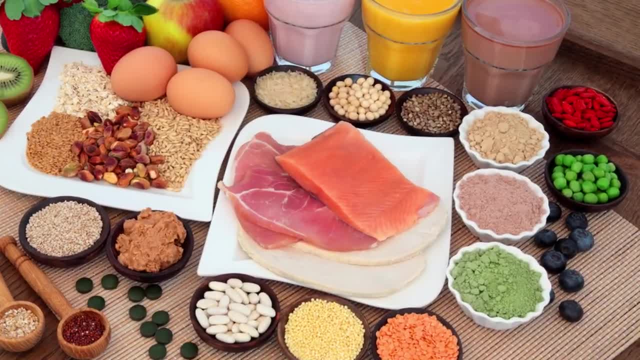 synthesis. They can be used to stimulate muscle protein synthesis. They can be used to stimulate in the body and must come from food. The reason leucine is singled out is it's the most effective one at stimulating protein synthesis, which is the process of repairing and building new muscle. 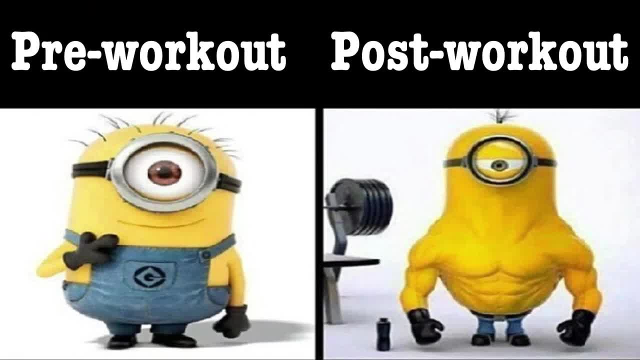 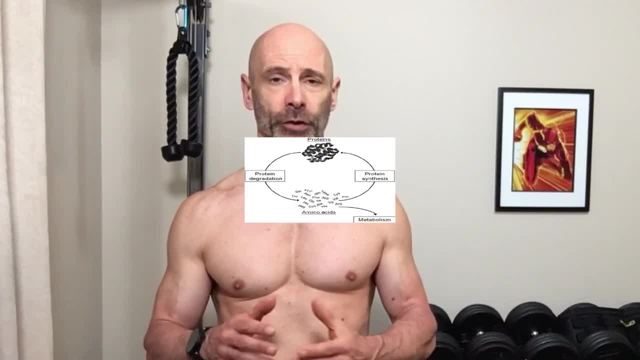 tissue. This doesn't just happen after our workouts. It's happening in our bodies all the time. It's a continual process called protein turnover, where the older and damaged proteins in the cells are removed- called protein degradation- and replaced with new proteins. 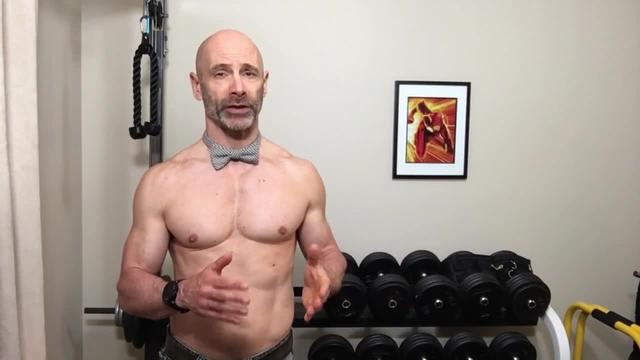 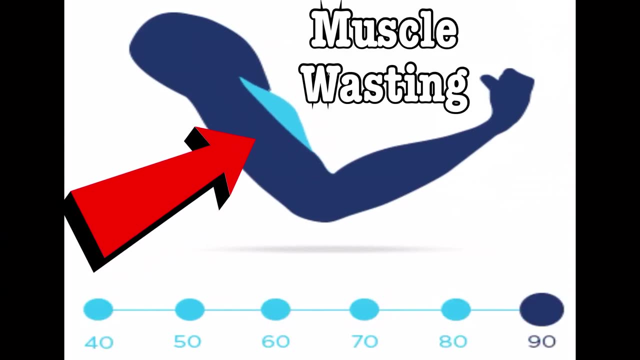 or protein synthesis. If the removal of these damaged proteins happens faster than the rate of protein synthesis, then we have muscle wasting. Another thing it does is enhance glucose and insulin homeostasis. Insulin and glucagon are hormones that work together to keep your blood. sugar levels in check. When these hormones aren't working properly, you'll get food cravings and you can even end up suffering from prediabetes and diabetes. So how much leucine should we be taking every day? To try and find this, I read a wide range. 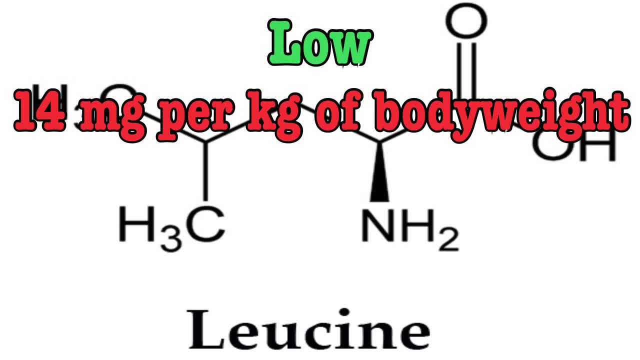 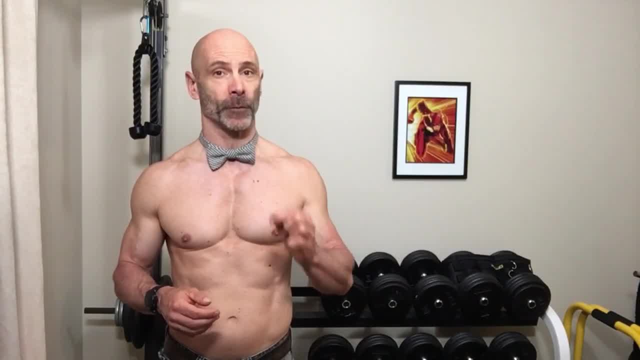 of recommendations, with the low end being about 14 milligrams per kilogram of body weight and the high end as much as 45 milligrams. The good news is, if you're taking in enough protein from high-quality food sources, you'll get all the leucine you need. 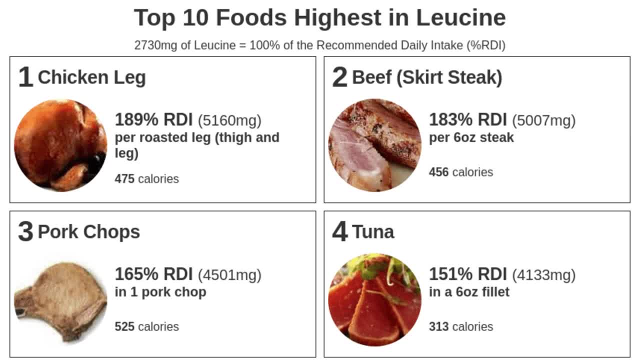 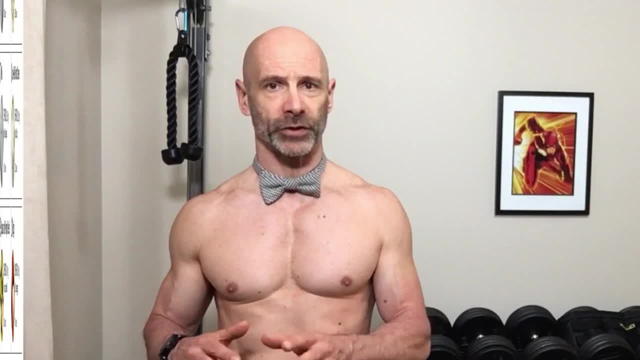 Meats top the list of foods high in leucine, with chicken, beef and pork leading the pack. Fish and dairy are also good sources. Nowadays, people are trying to cut back on their meat consumption. For those, navy beans are a great choice, having slightly more leucine per 100. 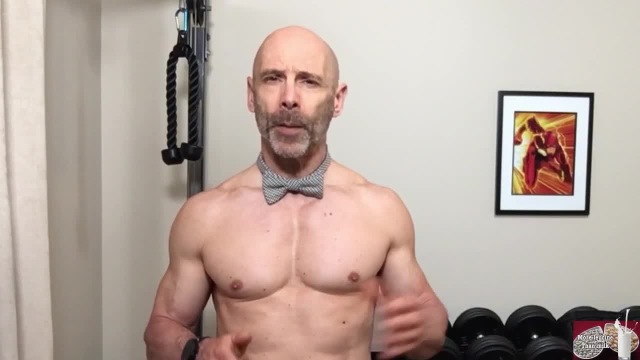 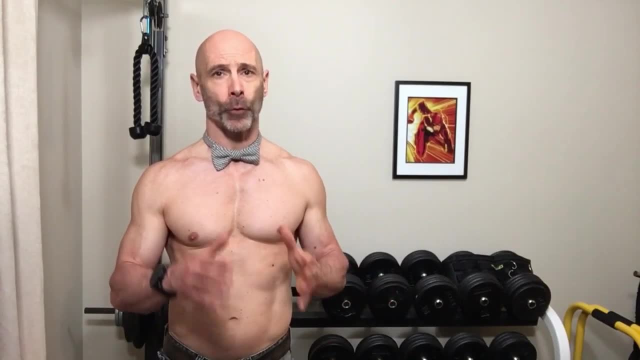 grams than milk and tofu has even more. Beans in general have a generous amount of leucine. The next step down from beans is nuts and seeds. These contain about half or less the amount of leucine found in beans, but it's still a reasonable amount. 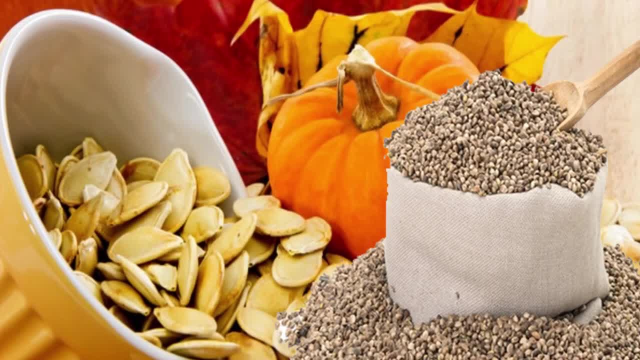 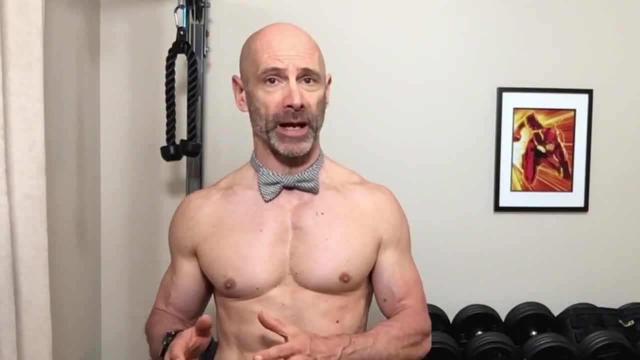 Pumpkin and squash seeds top the list, with hemp seeds, following close behind Walnuts, and pistachios head up the list for nuts. Now I don't want you to think I'm underestimating the importance of the other amino acids, and in particular the nine essential.